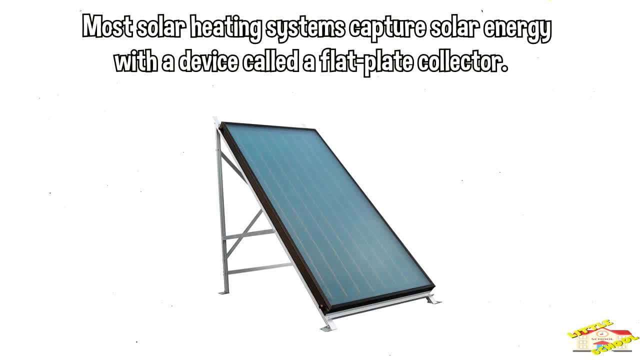 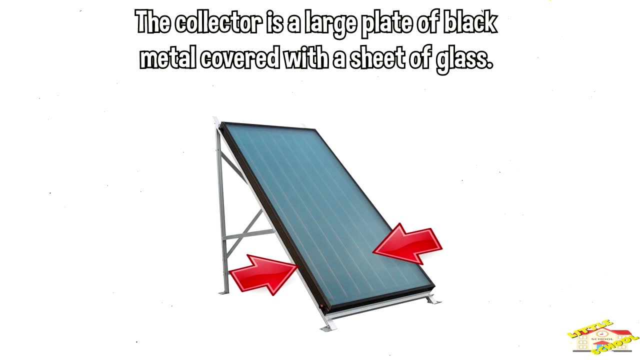 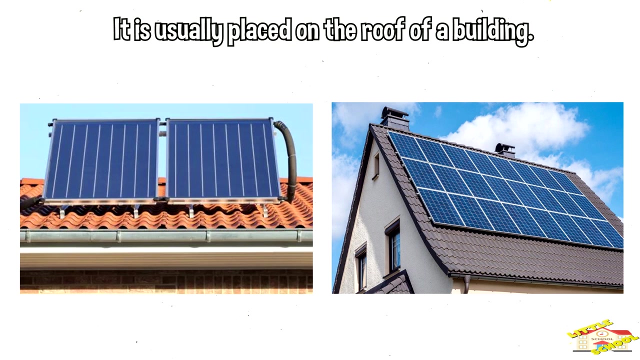 Most solar heating systems capture solar energy with a device called a flat plate collector. The collector is a large plate of black metal covered with a sheet of glass. It is usually placed on the roof of a building. The plate absorbs sunlight and uses it to heat air or 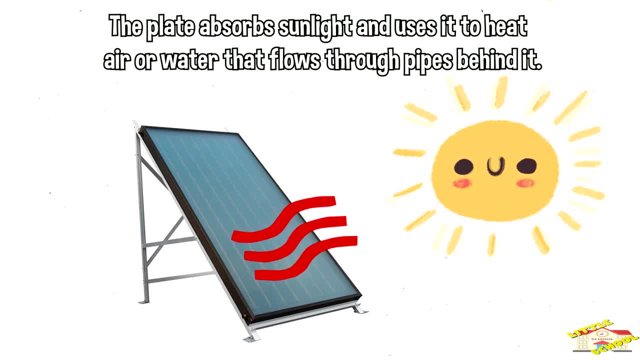 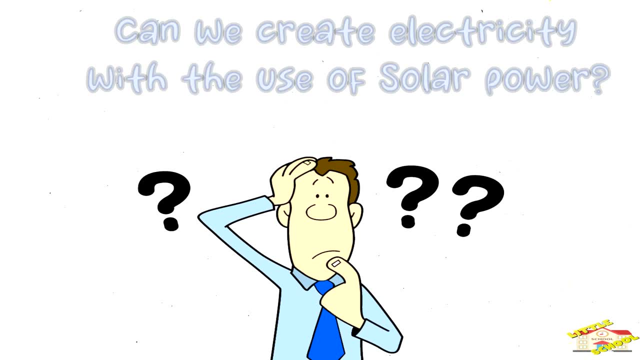 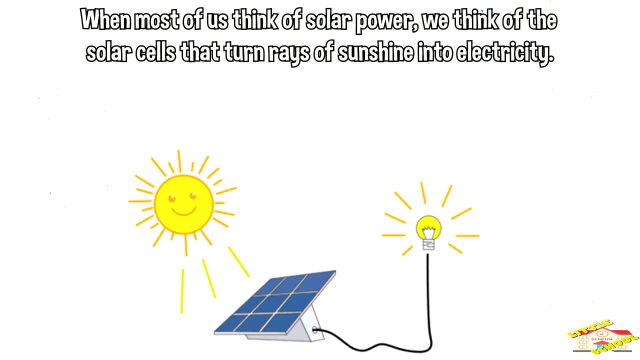 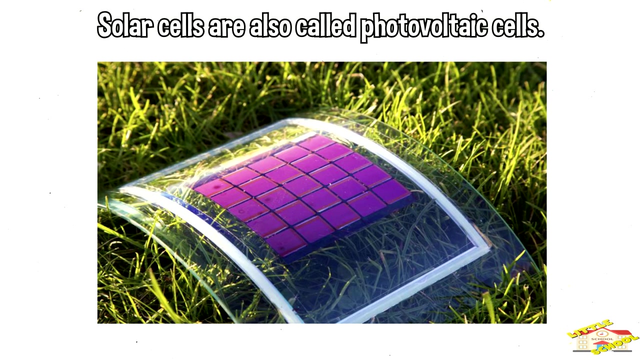 water that flows through pipes behind it. Can we create electricity with the use of solar power? When most of us think of solar power, we think of the solar cells that turn rays of sunshine into electricity. Solar cells are also called photovoltaic cells. The word photovoltaic. 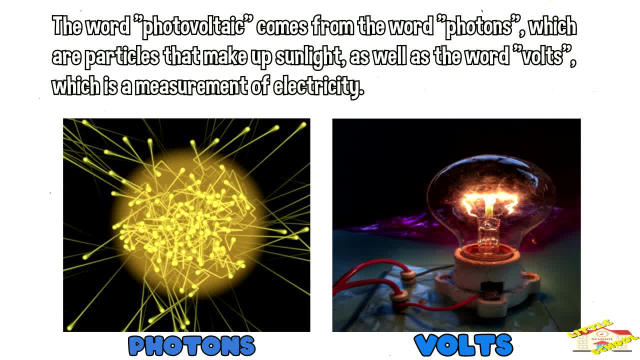 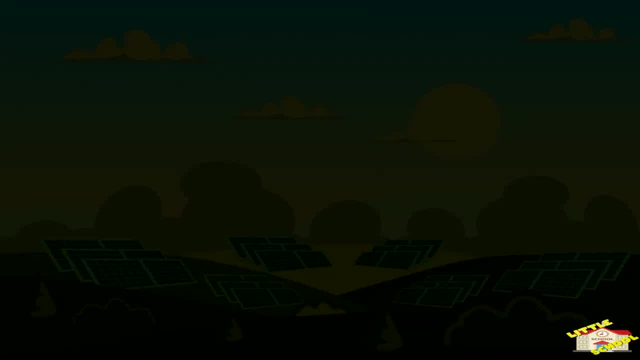 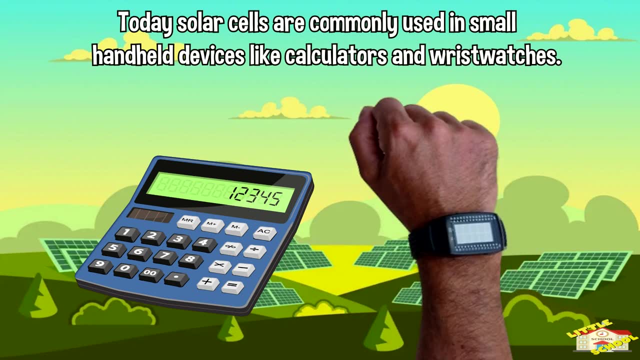 comes from the word photons, which are particles that are produced by the sun. Photons are particles that make up sunlight, as well as the word volts, which is a measurement of electricity. Today, solar cells are commonly used in small handheld devices like calculators and wristwatches. 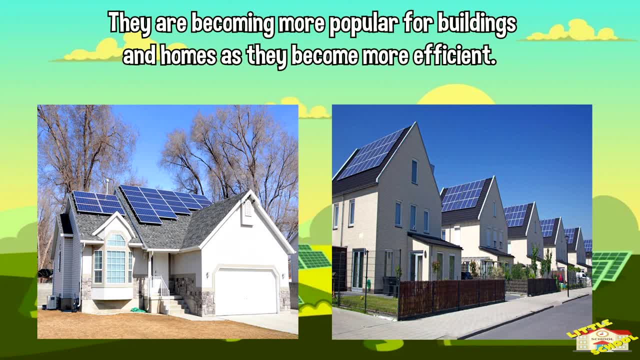 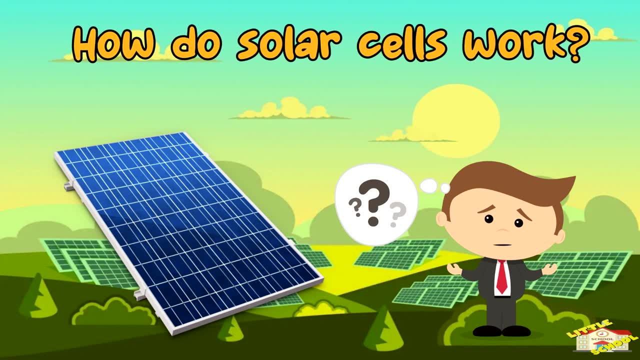 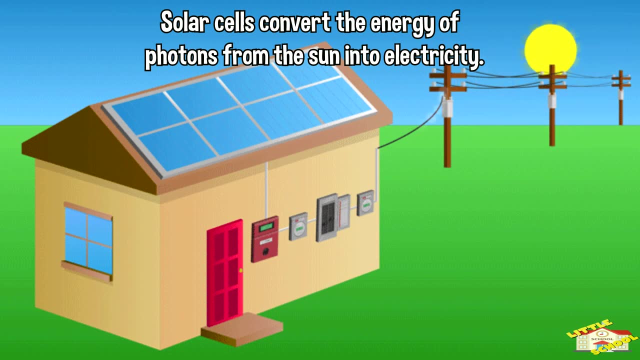 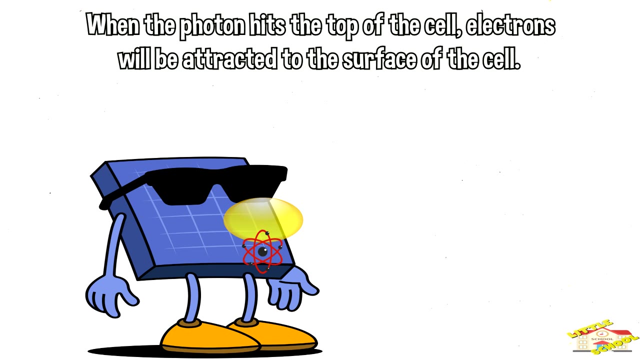 They are becoming more popular for buildings and homes as they become more efficient. How do solar cells work? Solar cells convert the energy of photons from the sun into electricity. When the photon hits the top of the cell, electrons will be attracted to the surface. 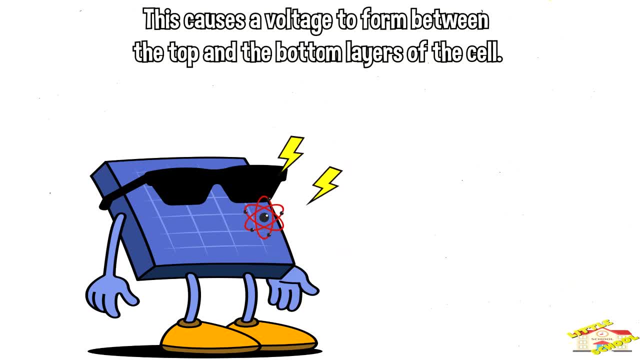 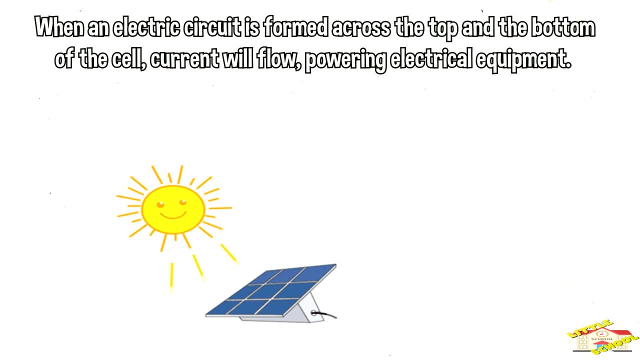 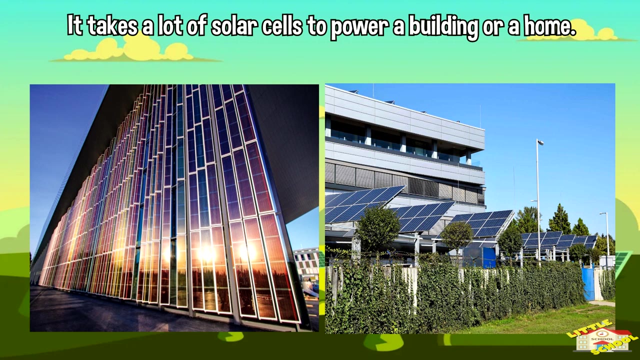 of the cell. This causes a voltage to form between the top and the bottom layers of the cell. When an electric circuit is formed across the top and the bottom of the cell, current will flow, powering electrical equipment. It takes a lot of solar cells to power a building or a home. 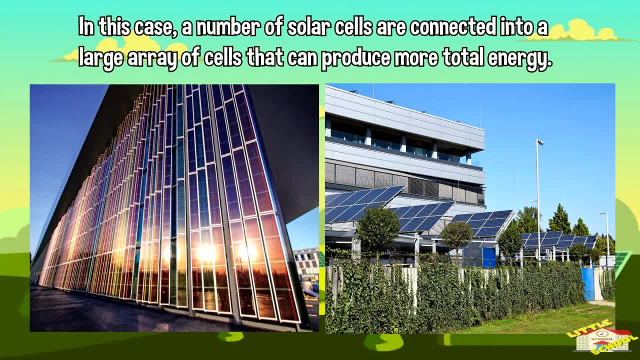 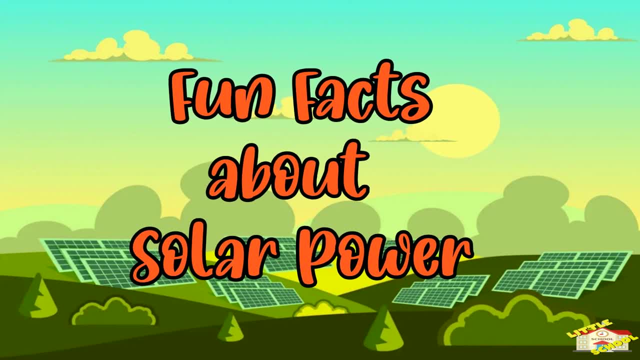 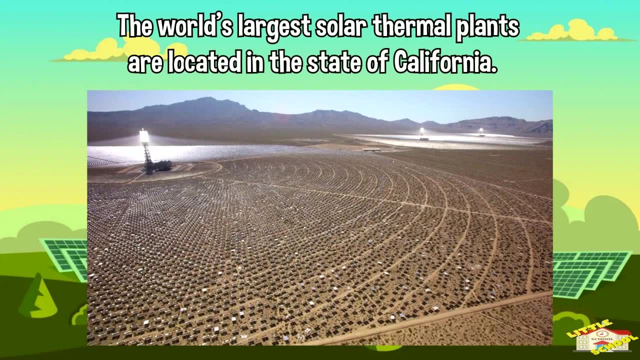 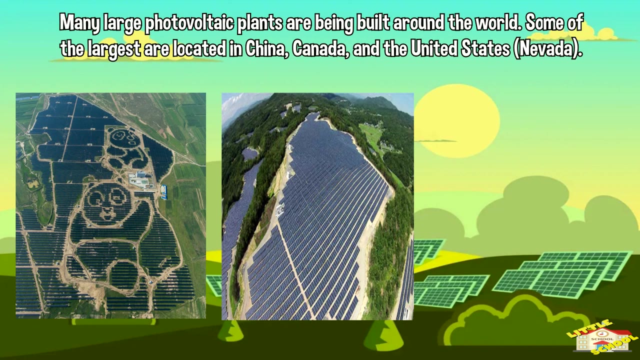 In this case, a number of solar cells are connected into a large array of cells that can produce more total energy. Here are fun facts about solar power. The world's largest solar thermal plants are located in the state of California. Many large photovoltaic plants are being built around the world.